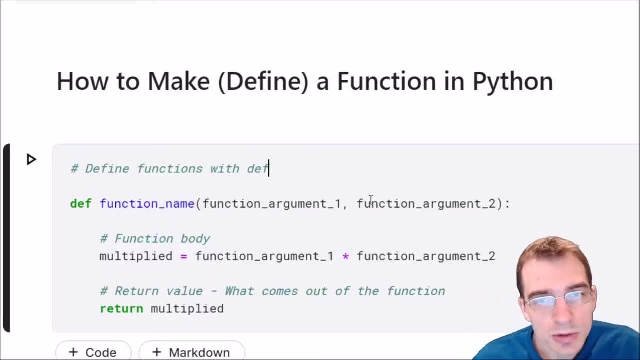 In this video we're going to learn how to make, also known as define, a function in Python. So to define a function, you start with this def keyword and then after that you put the name of the function. In this case we're calling it function name. Then you have some parentheses and within. 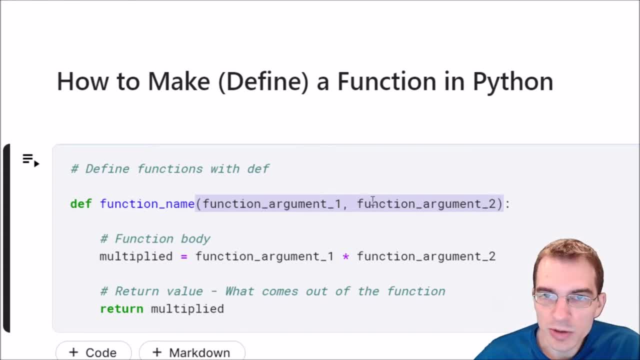 the parentheses you put any number of arguments you want to take into the function. Arguments are just bits of data that you are going to use within the function. So in this case we're going to take two arguments: one called function argument one, then comma function argument two. After you make 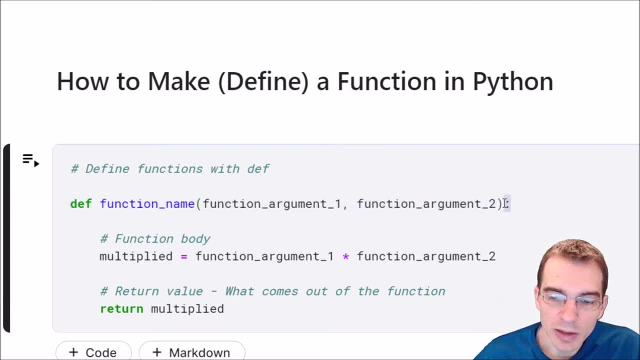 this whole definition statement. you put a colon and then everything that runs within the function is indented one level. So this part is the function body, because it's indented by one level, and all this function is doing is making a new variable called multiplied, which is these two arguments. 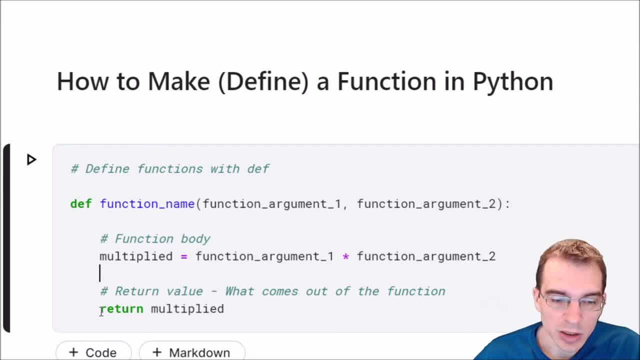 multiplied together, And then you see this final statement: here is return multiplied, So the return value within a function is what the function outputs. So in this case, this function- all it's going to do is take two arguments, multiply them together and then return the result. So when I actually run this, 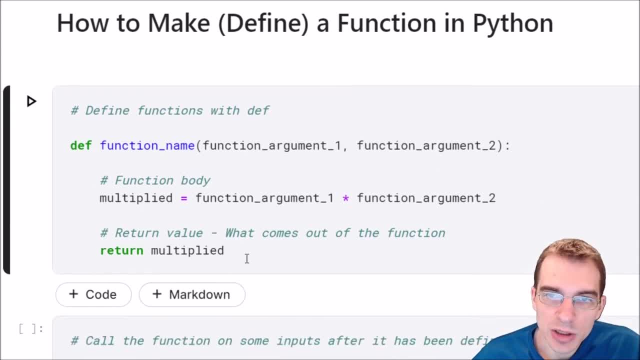 code block. here you'll notice that no output was actually generated. We didn't actually run the function yet. All this function definition does is define the function and then it's going to create the function itself. but we didn't actually run the function on any input. So we'll show how we 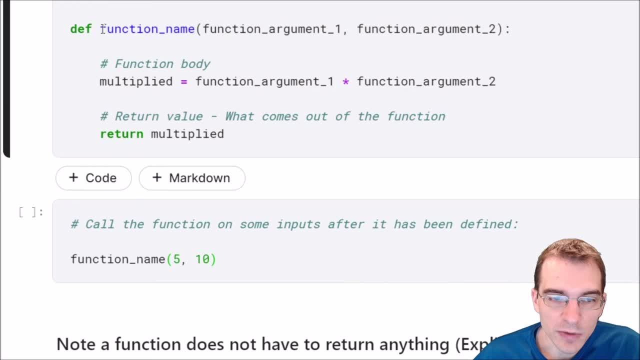 can do that. So below we'll take the name of our function. We called it function name. So to call the function we'll just say function name. Now it is defined, And then within the parentheses we put whatever arguments we want to pass into the function that correspond to each of the arguments we set up. 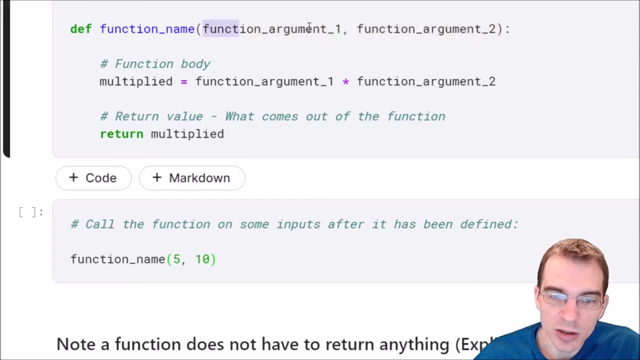 in the definition. So in this case our function requires two arguments and it's going to multiply those together. So we're going to call it function name And then we're going to put the function name And then we're going to. 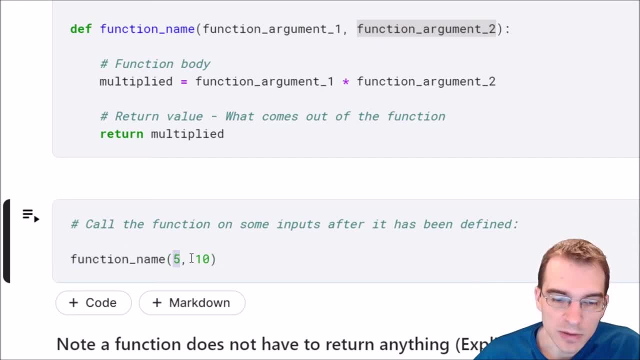 so we'll call it on function name 5- 10. so what this should do is pass these two numbers into the function, multiply them together and return the result. so let's run that and we can see that our function managed to do what it's supposed to do: multiply two numbers together. now it is worth. 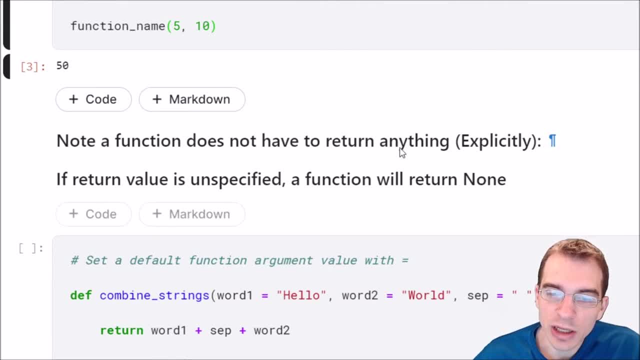 noting that a function doesn't technically have to return anything, at least explicitly. in our case we did say return two numbers multiplied, but we wouldn't have had to do that. we could have done something else in the function, like printed something or perhaps manipulated a list in. 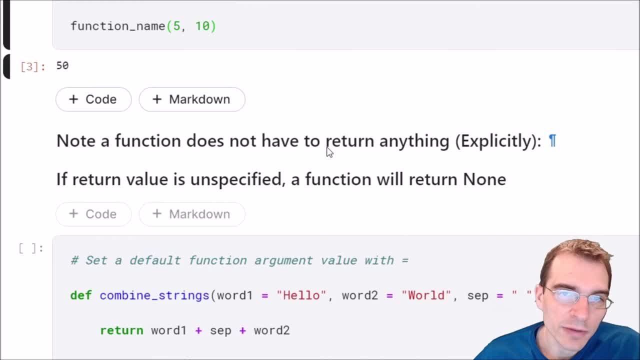 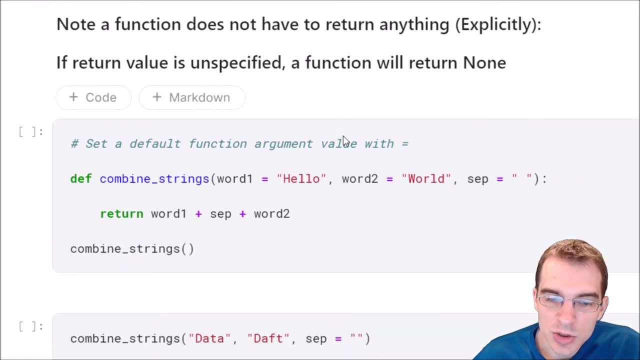 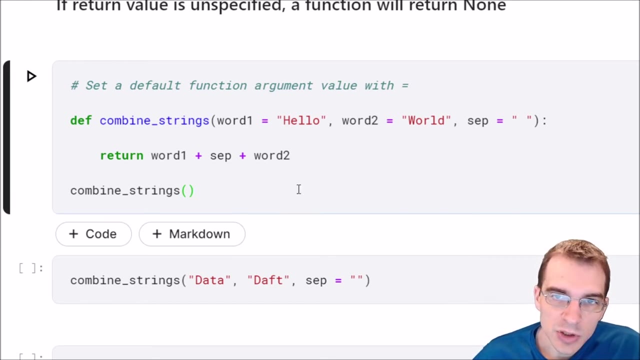 place and that wouldn't have a return value. if you do define a function that doesn't return anything explicitly, the function will return none by default. now one other thing that is worth mentioning: when you define a function, you can give the arguments a default value. that first. 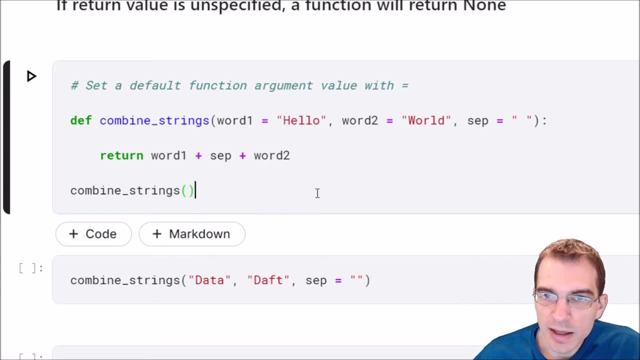 function we defined. they didn't have default values, so we had to pass in values when we called the function, otherwise it wouldn't have worked. but i'll give an example of making a function with some default values and then we don't need to supply arguments to those if we don't want to. 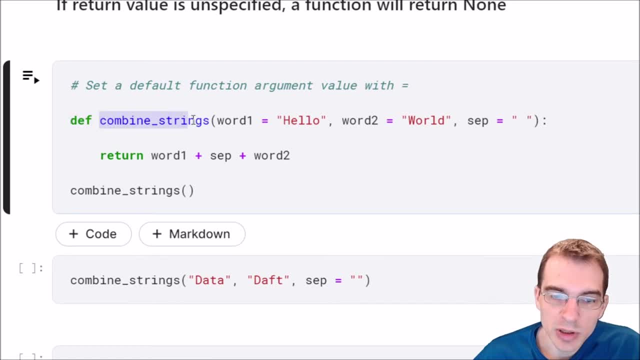 so we'll say def, define a new function. this one will be called combine strings and it's going to take some arguments but we're going to give them default values. so to provide a default value, we'll say the name of the argument, word one, but then we say equals hello. this equals hello means the. 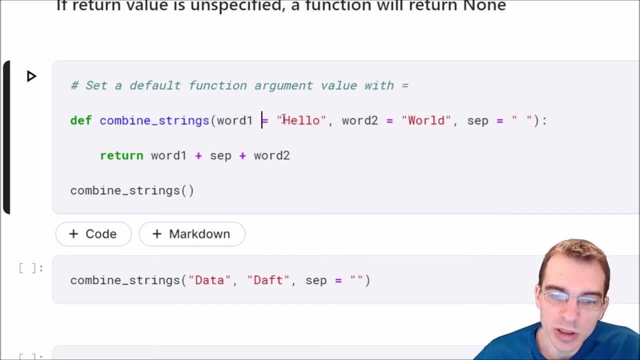 default value for this word. one argument is going to be the string hello. and again for word two, we're going to give that a default value of world. and then a third argument: sep- separator. we're going to give that a default value of just a space, and what this function is going to do, it's going to take that word one, separator, and word two, and 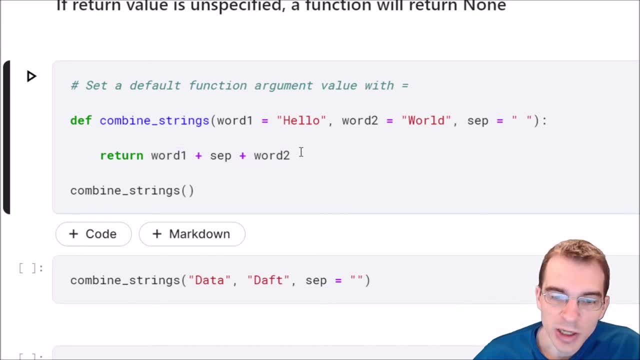 then return the result with all those added together. so with python strings that's basically just taking two words, adding them together and putting a space in the middle. so if we define that and then we'll run combined strings, notice when we're running combined strings. in this case we're just 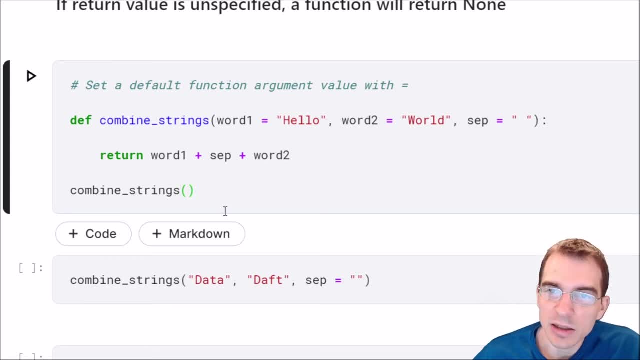 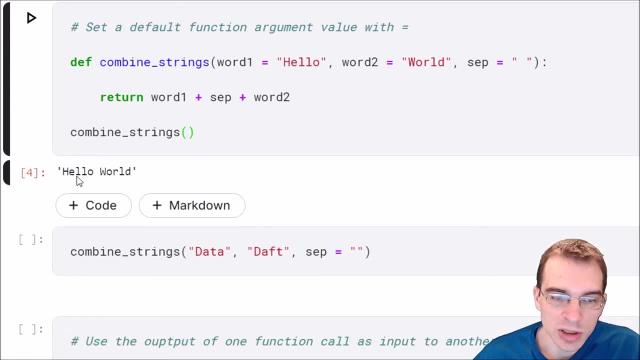 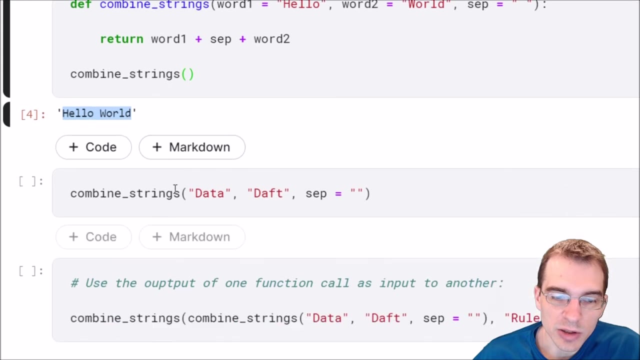 putting the parentheses here because we don't need to add any extra arguments to this. we already supply defaults, so let's run this on the defaults. if we just use the defaults, it just prints hello world with the space in between it. but we could, if we wanted to do something without the defaults.